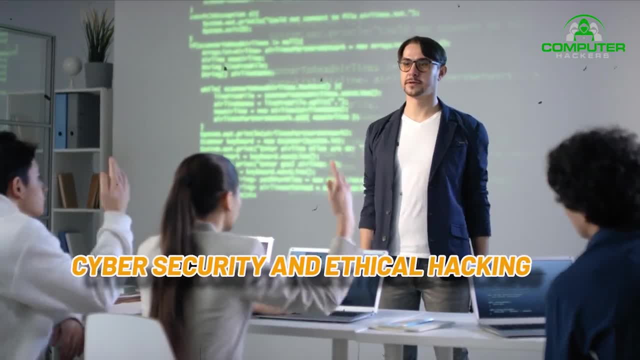 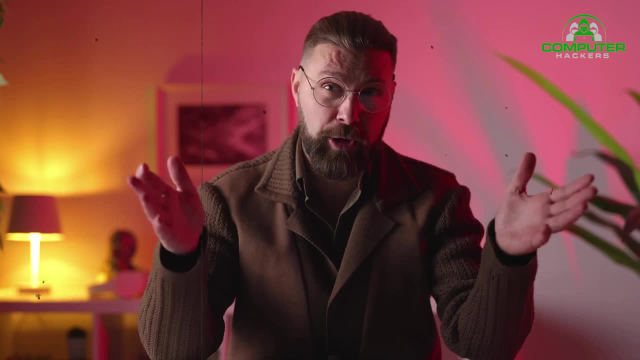 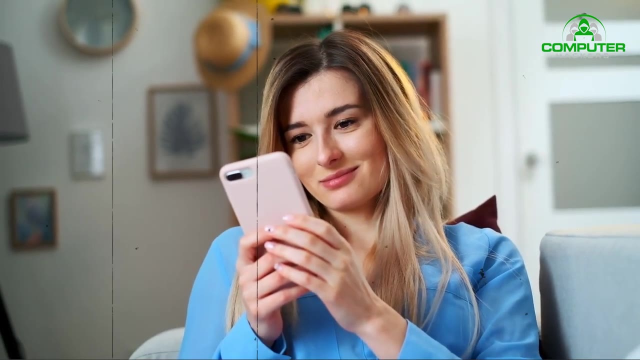 Difference between cyber security and ethical hacking. Hello friends, In today's video, we're going to be discussing the difference between cyber security and ethical hacking. By the end of this video, you will have a better understanding of the two concepts and be able to make more informed decisions when it comes to your online security. 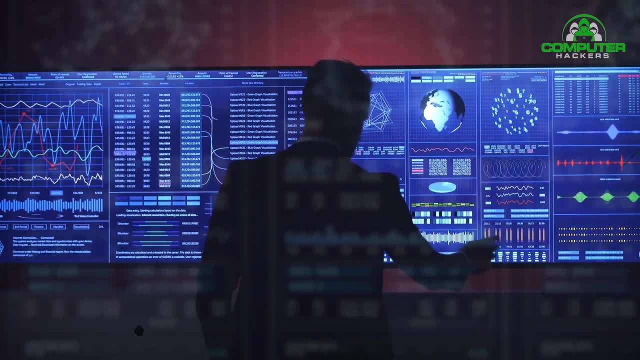 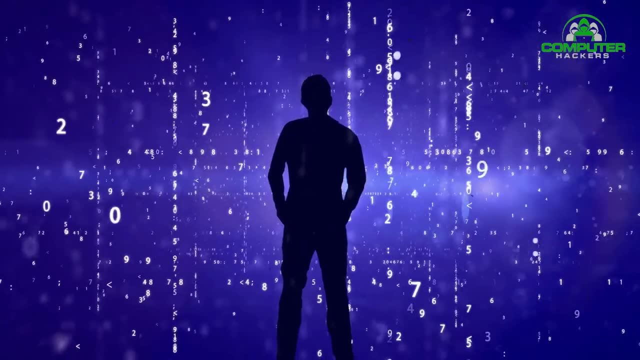 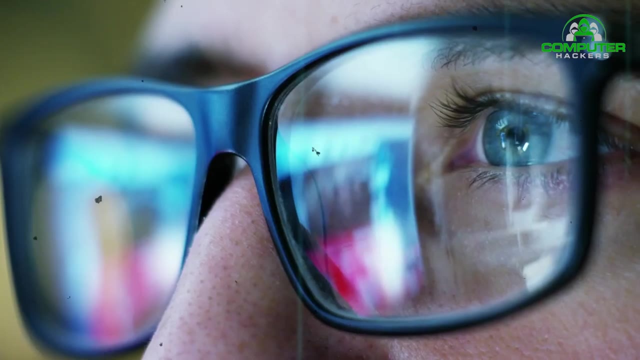 Whether you are a business owner or an individual who uses the internet regularly, it is important that you understand these terms so that you can take the necessary precautions to protect yourself and your data. What is cyber security? Before elaborating upon the difference between cyber security and ethical hacking, 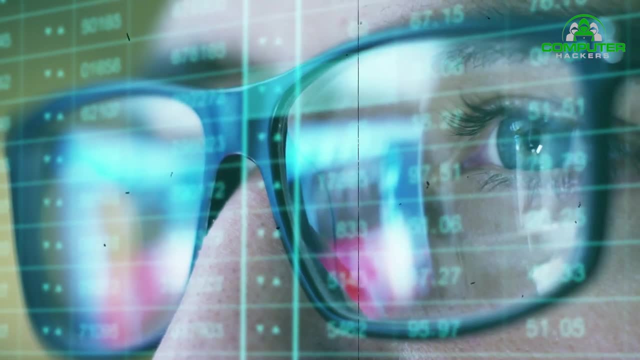 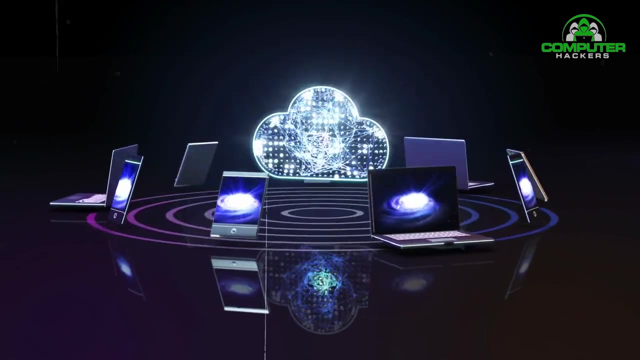 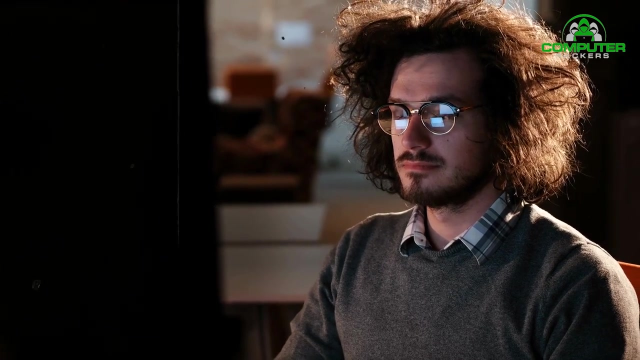 let's first understand what cyber security actually means. Cyber security can be defined as the practice or a process designed in order to defend networks, computers and data from damage, malicious attacks or unauthorized access. It is a combination of skills and tools which provide security to its users from. 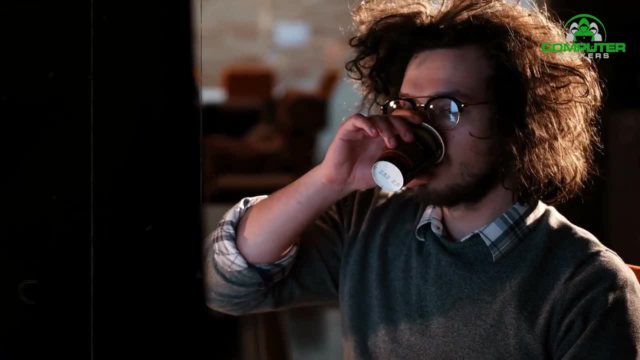 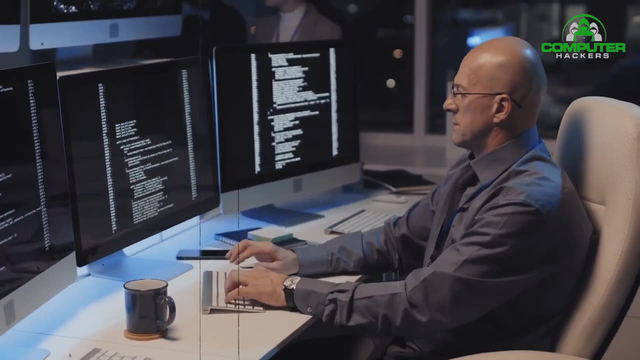 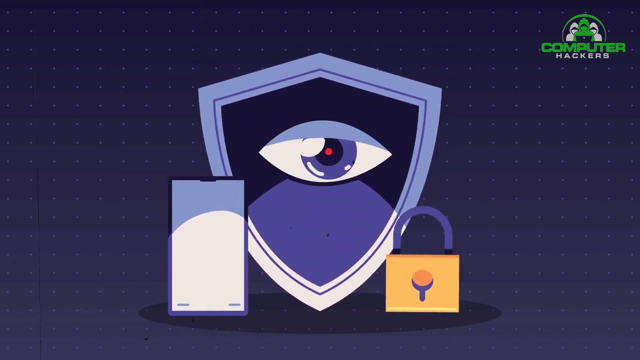 many attacks on their data devices or programs. Cyber security is becoming more and more important day by day. Every organization, whether government or private, stores unprecedented amounts of data, which is extremely crucial for that organization and needs proper security against any cyber threat. The global cyber threat continues to evolve at a rapid pace and every organization needs to. 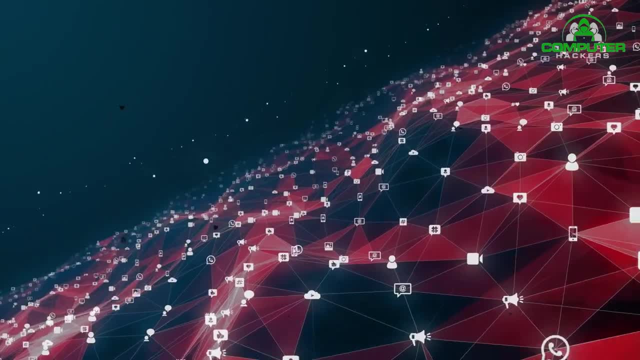 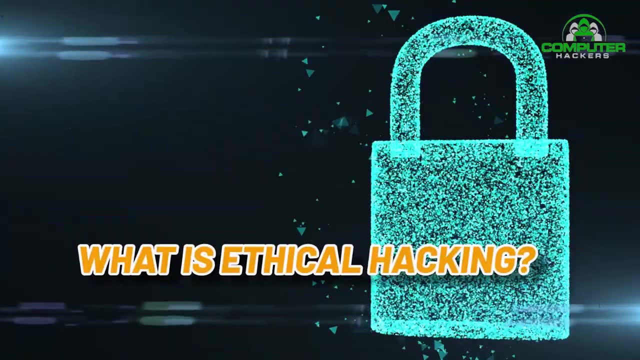 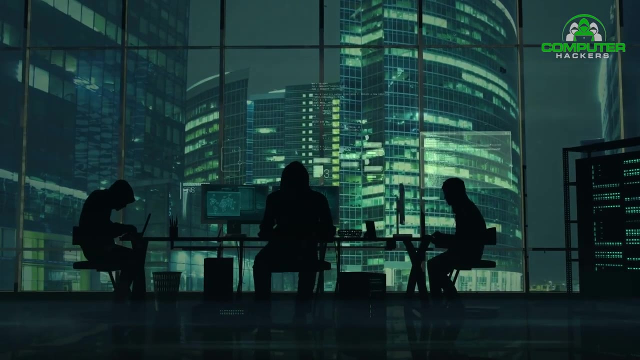 take appropriate steps in order to protect their sensitive information, especially those organizations that are involved in safeguarding national security data or other sensitive data. What is ethical hacking? Ethical hacking is a part of cyber security and can be defined as the process of testing the system against all possible security breaches and solving any vulnerabilities in the system before any malicious attack even happens. 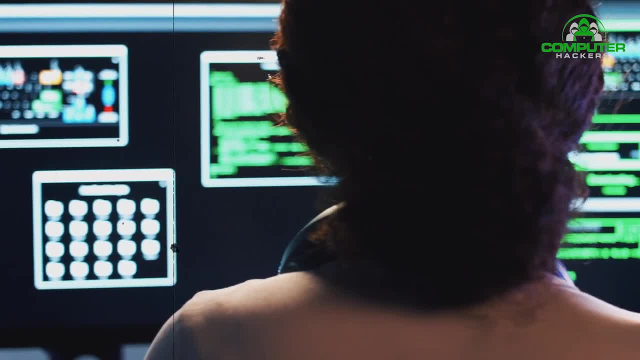 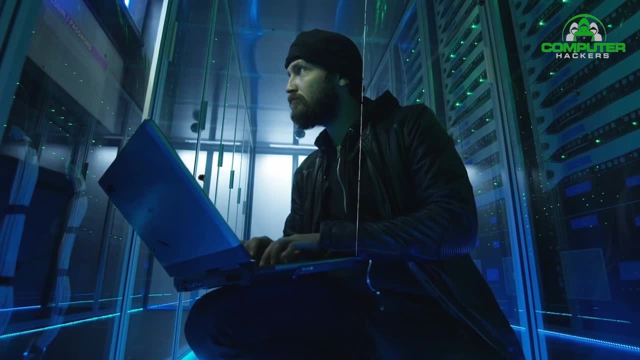 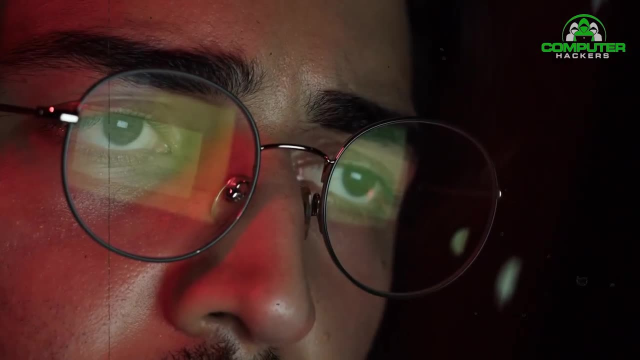 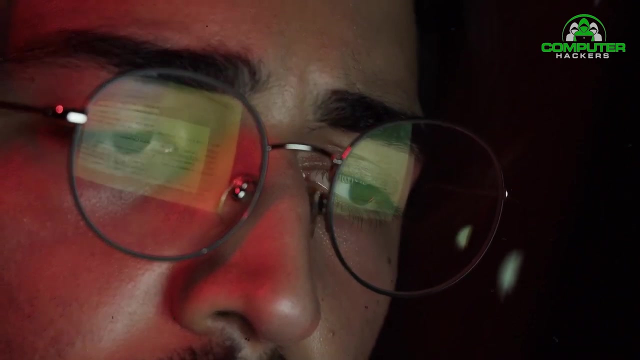 Hacking is illegal, but ethical hacking is the authorized practice of bypassing system security. to identify any potential data threat, Ethical hackers try to examine the systems to pinpoint the weak points in that system that malicious hackers can exploit. Ethical hackers are also referred to as white hat hackers, as their work involves the same as black hat hackers, but ethical hackers don't intend to harm anyone through their actions, but only protect their systems. 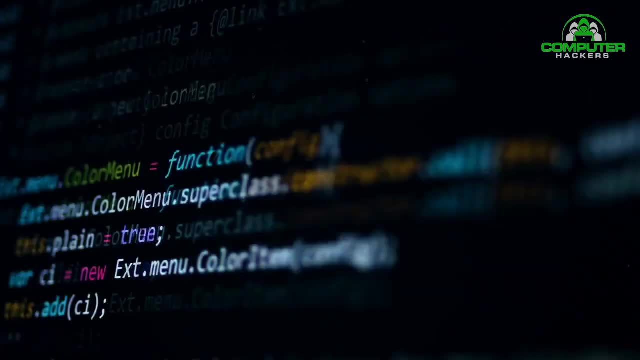 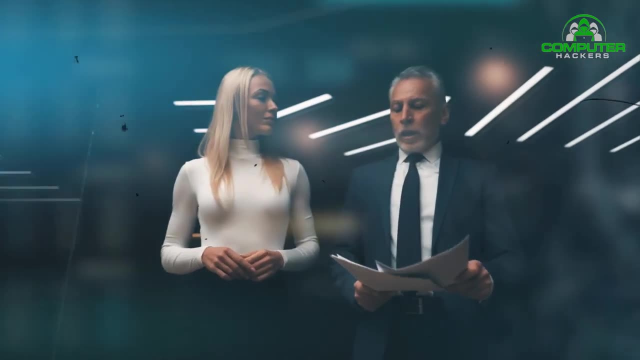 Suppose that your website or application contains sensitive data about your customers. Malicious hackers can misuse this data for wrongful purposes, So you will need an ethical hacker to prevent any of such malicious attacks from even happening. and if it happens, then the ethical hacker will perform the necessary actions. 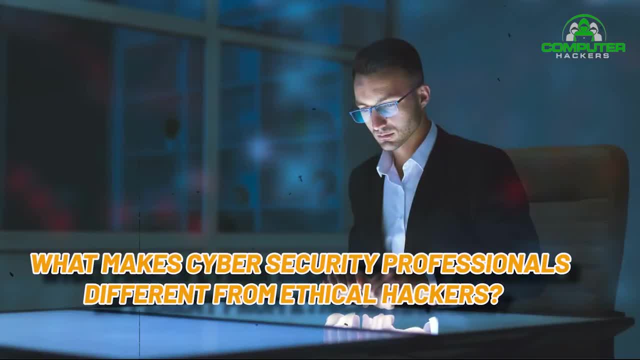 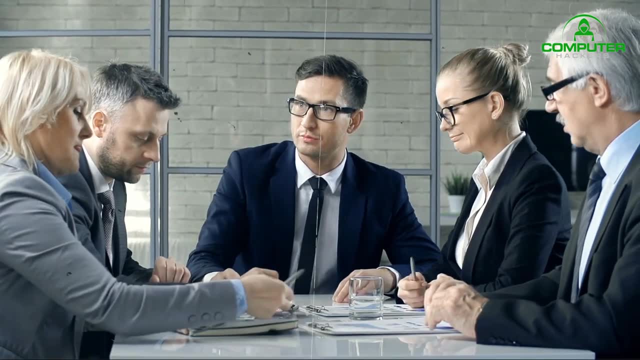 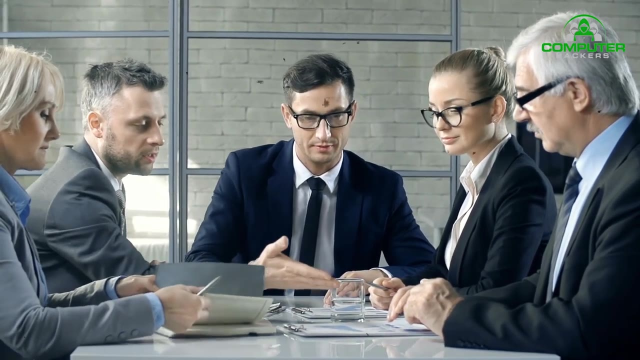 required to stop the attack. What makes cybersecurity professionals different from ethical hackers? To further understand the difference between the cybersecurity and ethical hacking, and which one's better for you, let's take a look at what role you can expect to play as an ethical hacker or cybersecurity professional. What does ethical hacker do? 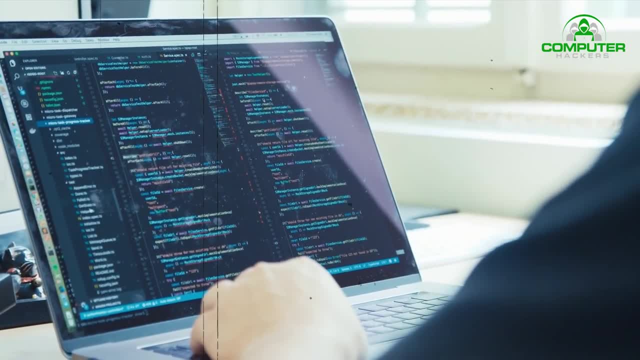 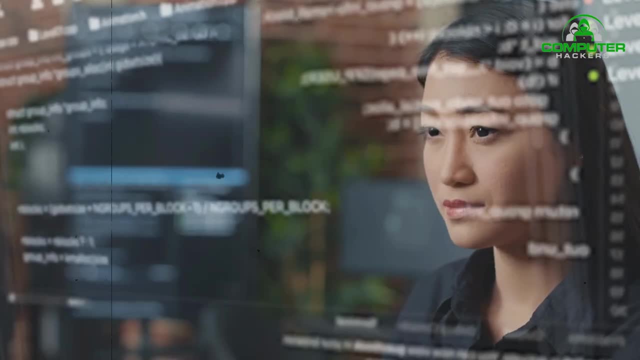 The job of an ethical hacker is to hack inside the system with consent or permission of the owner and provide a report about how it got hacked and track the main sources. Here are the key responsibilities that separate an ethical hacker from a cybersecurity expert: Evaluate the 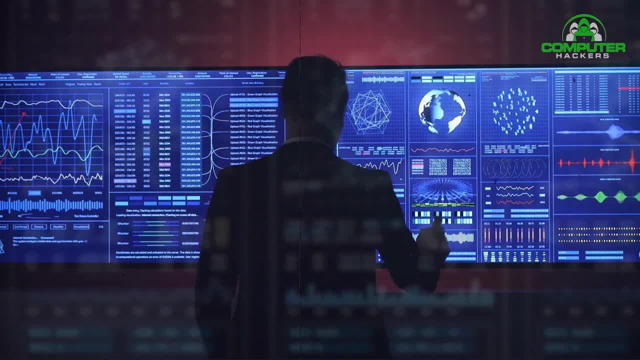 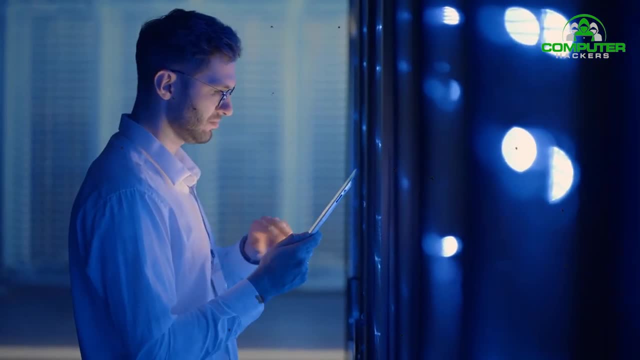 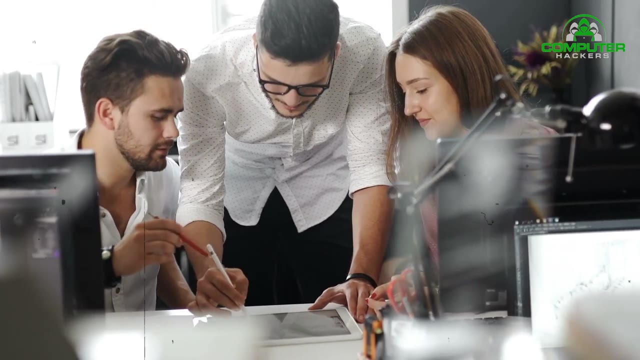 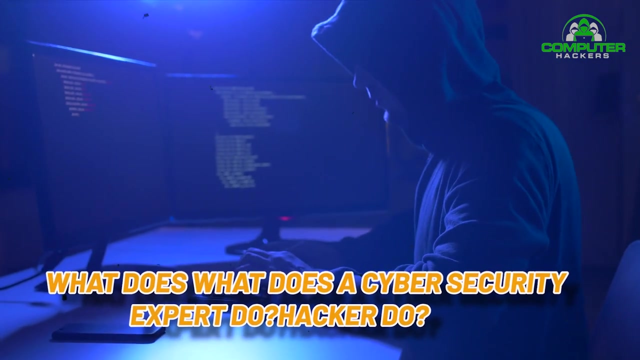 performance of the system. Test the security system. Suggest solutions to enhance the security system. Inform the organization about any malicious attack. Find weaknesses in the security system. Use appropriate techniques of hacking. Generate reports after finding vulnerabilities in the security system. What does a cybersecurity expert do? Cybersecurity experts work on securing. 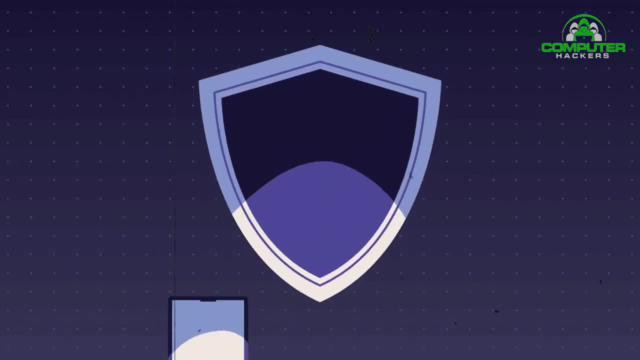 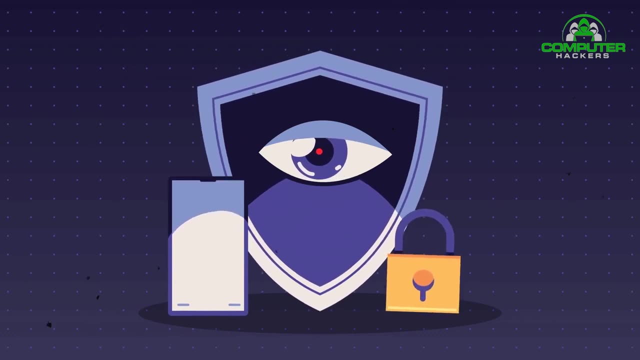 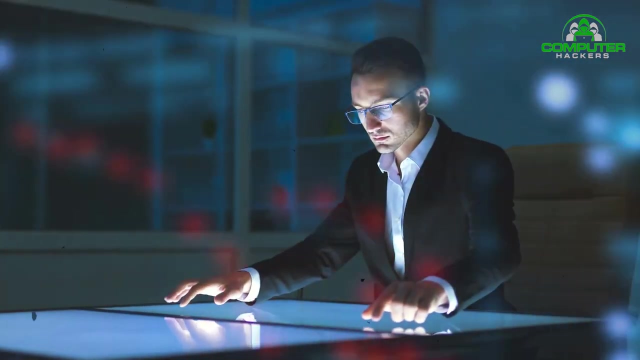 information systems by monitoring, detecting, analyzing and responding to security experts. In simple terms, they work on protecting systems against cybersecurity risks, vulnerabilities and threats. Here are the key responsibilities of a cybersecurity professional: Improve the security system. Maintain the security system by keeping it updated regularly. 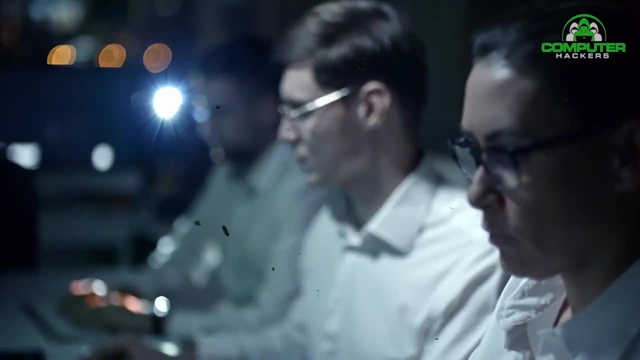 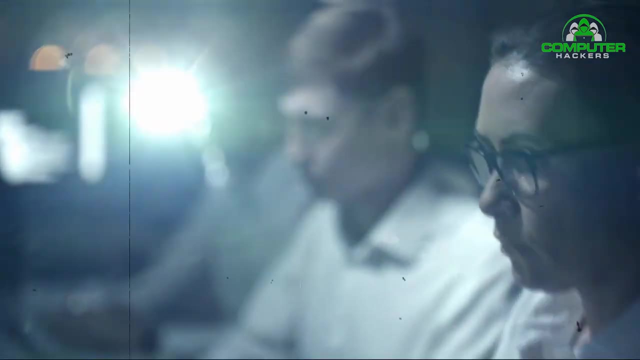 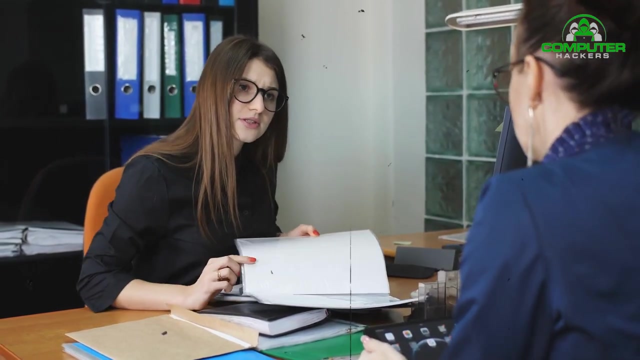 Work on IT teams in order to protect the integrity of a business's network and data, Analyze the security system and provide suggestions regarding the same to the organization. Career in cybersecurity and AMP ethical hacking. Due to the increasing threats of attacks on data and misuse of data, the field of cybersecurity is becoming bigger than ever and is rapidly increasing. 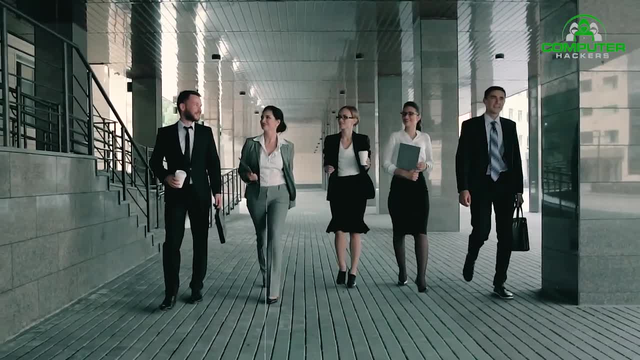 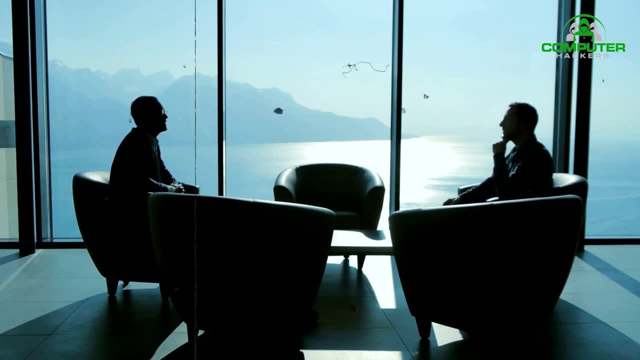 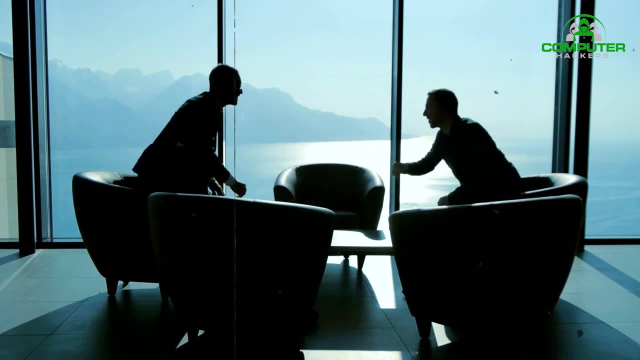 The demand for cybersecurity experts is more than ever, and the number of professionals in this field is getting shorthanded in fulfilling the demand. Therefore, there is a shortage of skilled professionals in this field. so if you have any interest in information technology or ethical hacking, then there is no better time than this to enter the field. 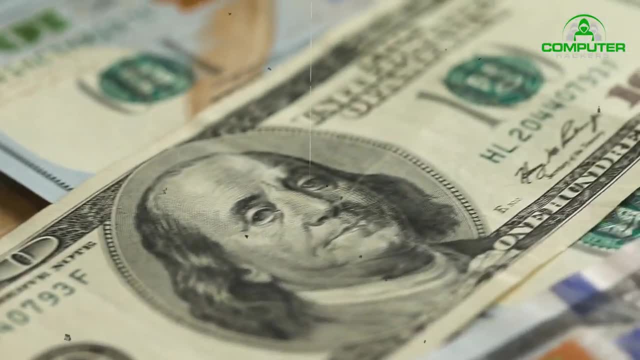 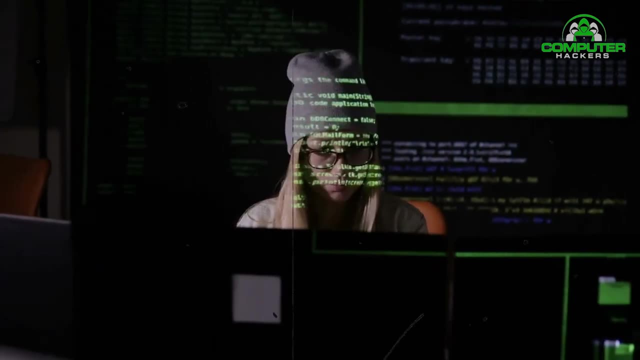 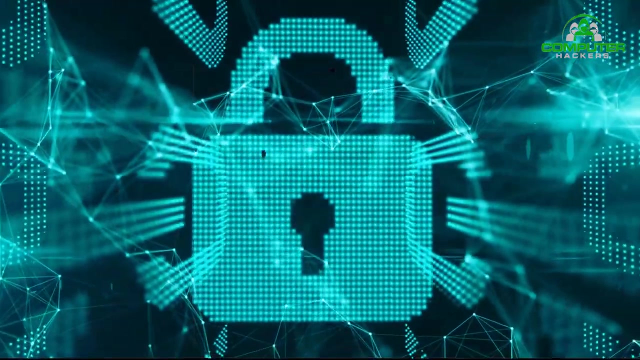 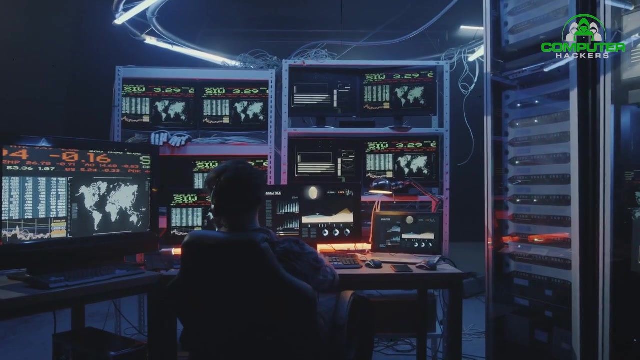 The cybersecurity market is predicted to become a $170 billion market in the near future itself. Why is cybersecurity important? Cybersecurity is important for several reasons. First and foremost, it's essential for protecting businesses from cyber attacks. These attacks can involve anything from stolen data to crippling systems that impact the entire business. 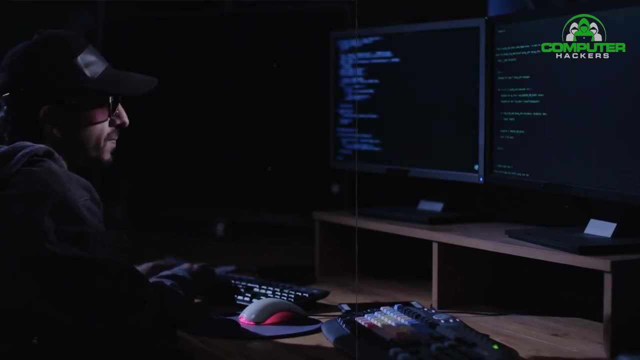 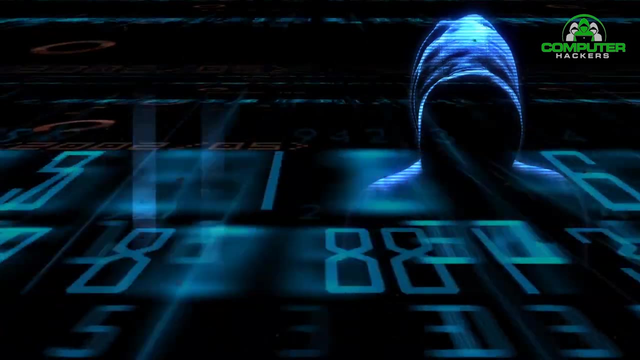 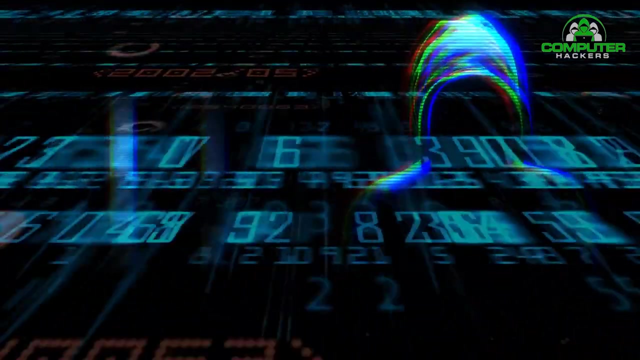 Cybersecurity is also important for safeguarding personal information, as well as protecting critical infrastructure like the power grid or the financial system. Second, cybersecurity protects companies from legal liability. If a company is hacked and data is stolen, the law often holds the company responsible, even if the hackers were not actually from that company. 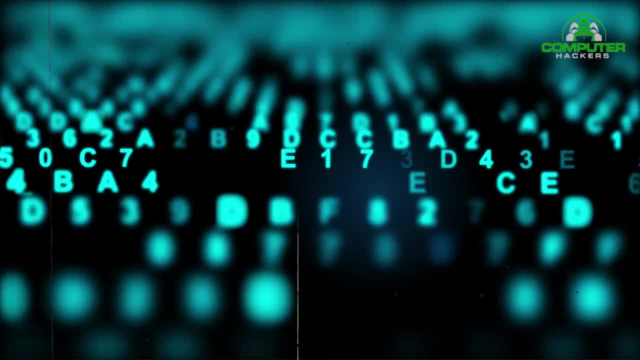 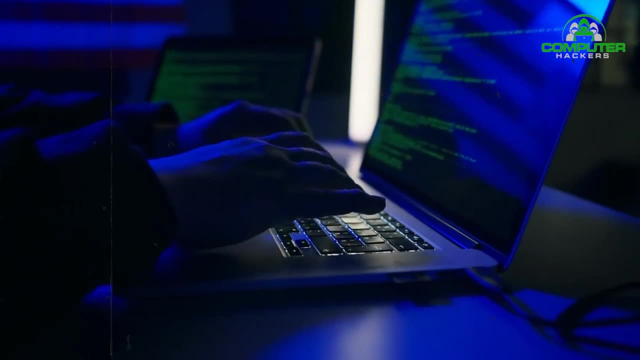 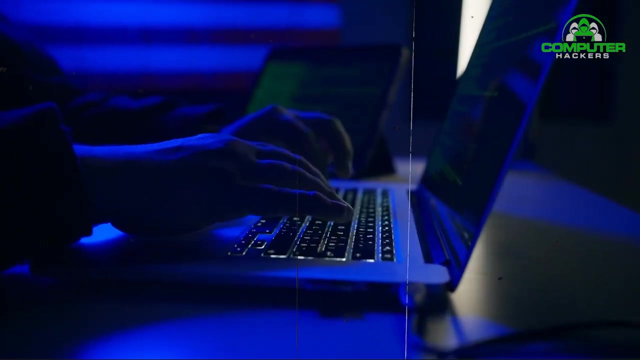 Cybersecurity also helps protect companies against lawsuits related to environmental damage or product defects. Finally, cybersecurity protects companies against government investigations and accusations of wrongdoing. By ensuring that their systems are properly protected against hacking and data breaches, companies can avoid embarrassment and potential legal problems. 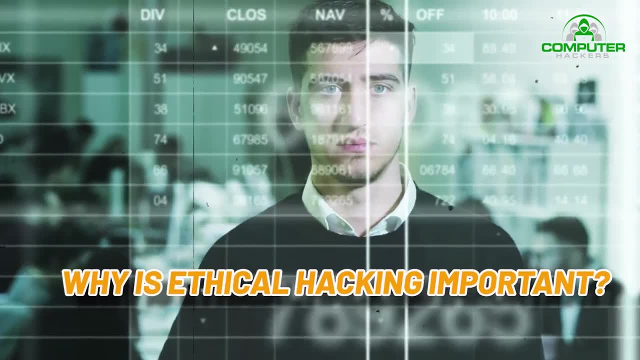 By ensuring that their systems are properly protected against hacking and data breaches, companies can avoid embarrassment and potential legal problems- legal problems down the road. Why is ethical hacking important? Ethical hacking is a process of testing the security of a system or network by attacking 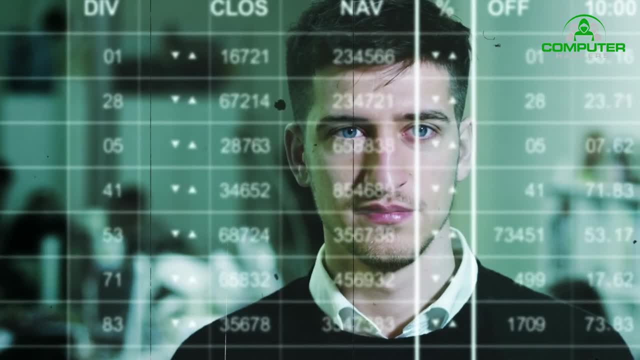 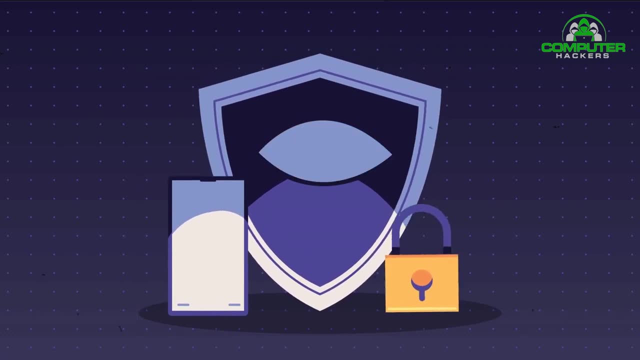 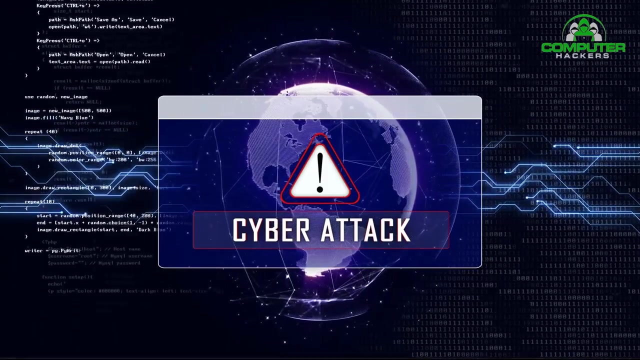 it and trying to find vulnerabilities. By doing this, you can help to protect the system from unauthorized access, destruction or theft. The benefits of ethical hacking are manifold. Not only does it improve the security of systems and networks, but it also helps to uncover. 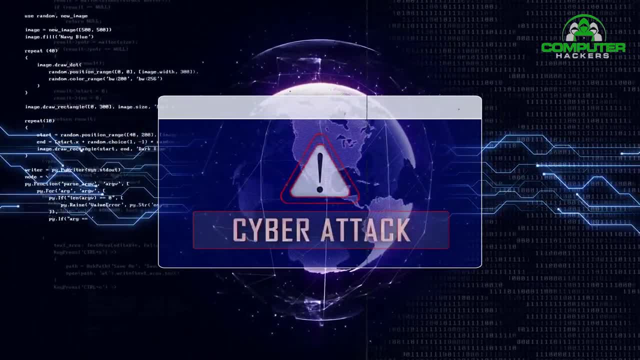 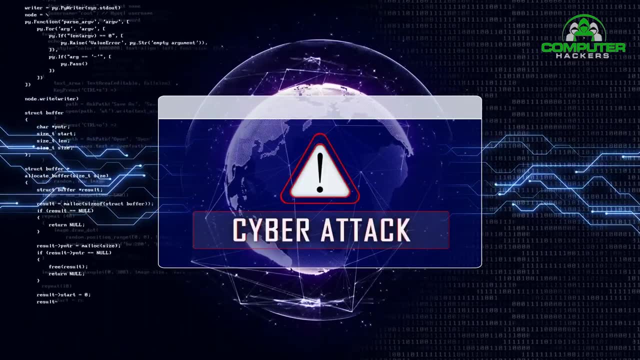 potential problems early on, in order to prevent them from becoming bigger problems down the line. Additionally, ethical hacking can also help identify any malicious behavior that might be taking place on those systems. If you're interested in getting started in ethical hacking, there are plenty of resources. 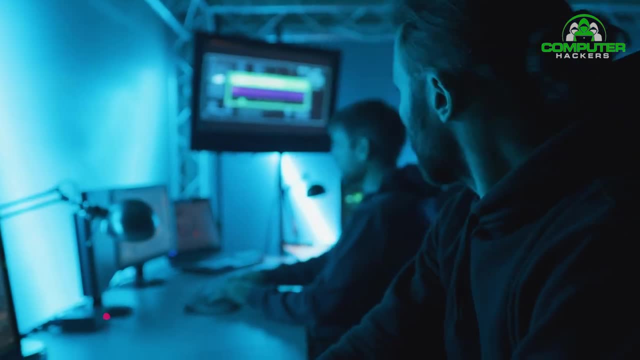 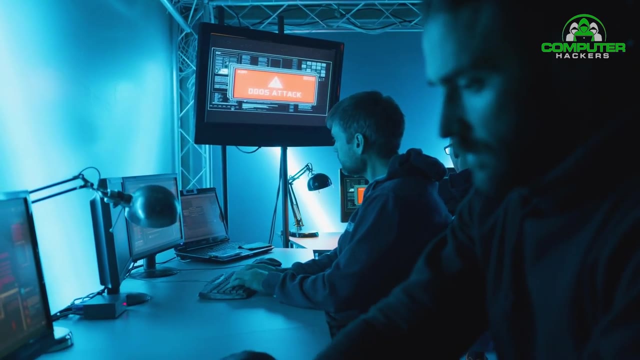 available online. One good starting point is the Ethical Hacking Academy website. They have a wide range of tutorials and scripts that will teach you everything you need to know about this fascinating field. I hope you guys surely like and enjoy our video. make sure to subscribe to our youtube. 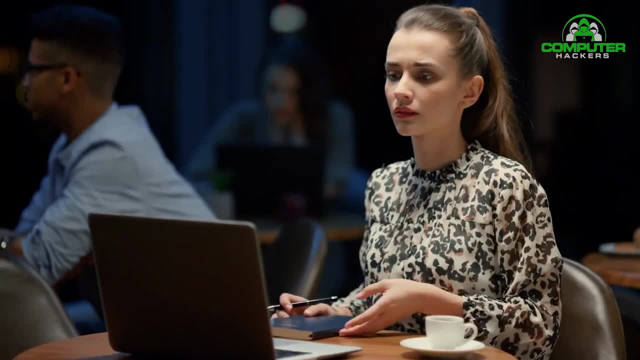 channel and hit the bell icon for upcoming videos. Thanks for watching.